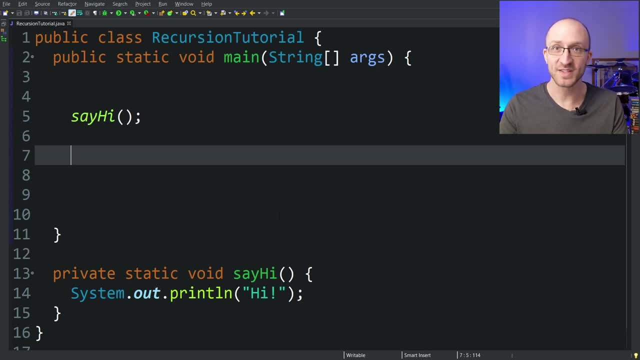 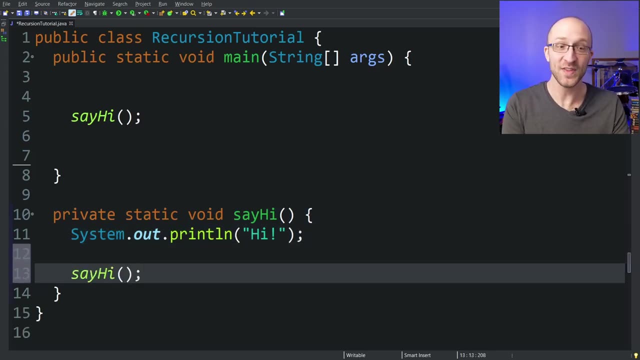 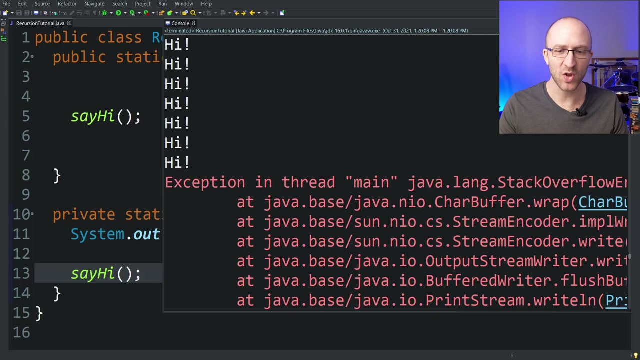 Remember, all recursion is is when a method calls itself. So all we have to do to make this method recursive is call: say hi from within this method. Okay, so it looks like it printed out hi a zillion times before eventually blowing up with a stack overflow error. So what exactly? 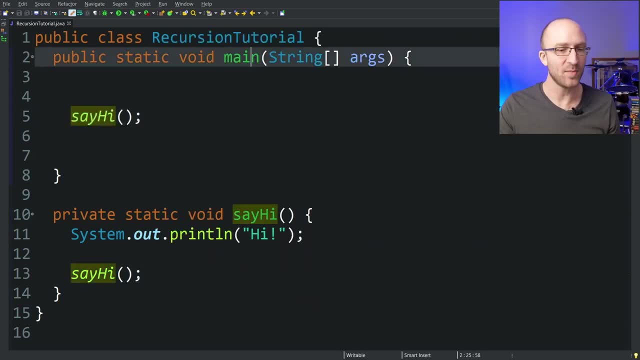 happened there? Well, when we first call say hi from our main method, it jumps into this say hi method and prints out hi. But then it makes a mistake. It prints out hi from within this method, A recursive call to itself. the say hi method calls the say hi method, And then that run of. 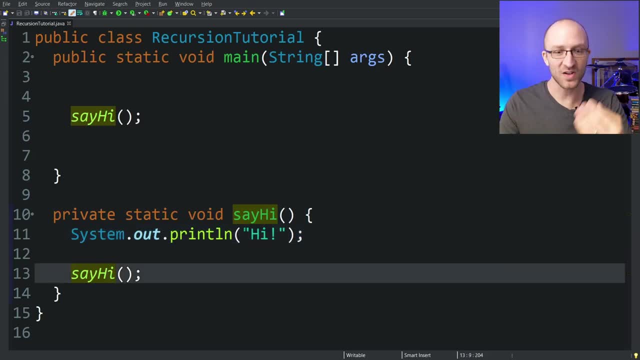 the method starts, it prints out hi and then it recursively calls, say hi again, So it kind of looks like this would just keep going on and on forever right. Kind of like if your program was stuck in an infinite loop, which you've probably run into before, where your program just keeps. 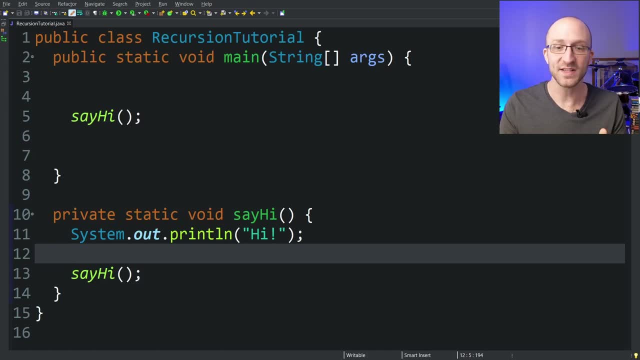 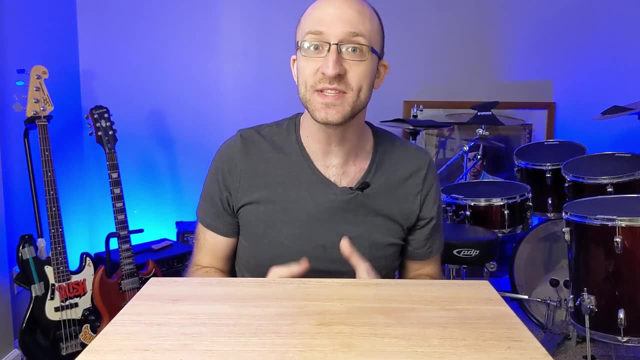 doing the same thing over and over again and never stops. But in this case, our program does stop when it runs into a stack overflow error. Why do we get this error? So here's what's happening: While your Java program is executing, every time it enters a new. 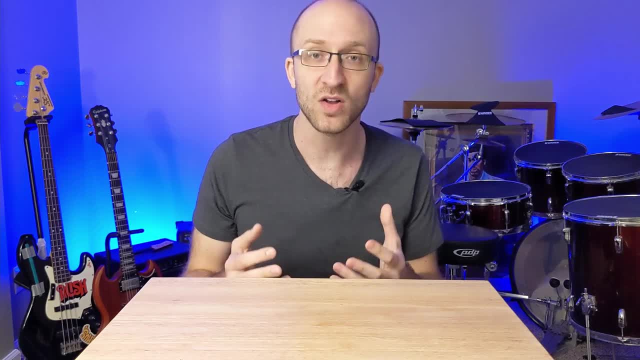 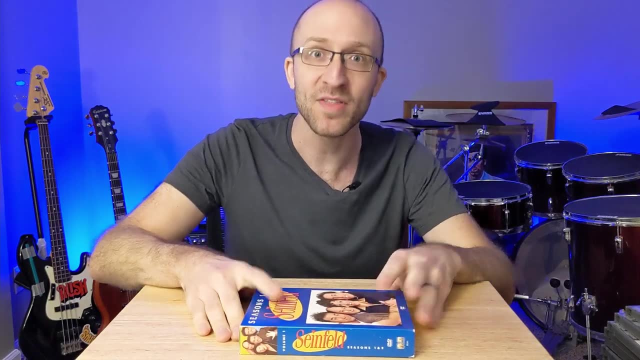 method, it puts the information for that method on something called the call stack. So at the beginning of your program when your main method starts, Java puts all the information for the main method onto the call stack. That information includes things like the name of the method. 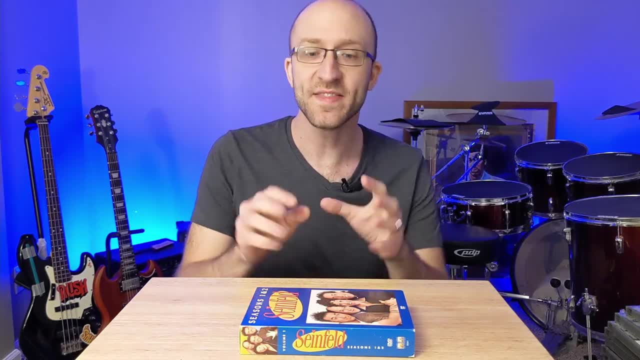 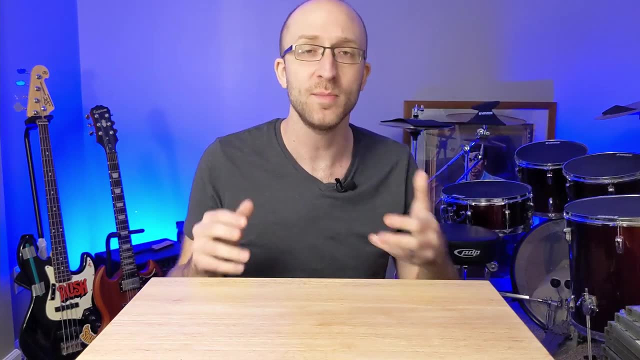 references to any variables that were passed in things like that. Once that method finishes and your program leaves the method, Java takes the information for that method off of the call stack Because it doesn't need it anymore. And if that method was the main method at the bottom of the call? 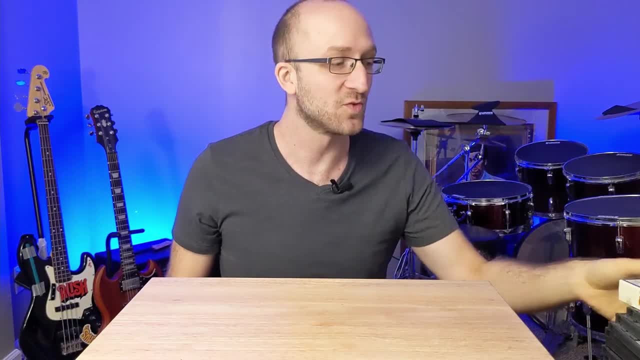 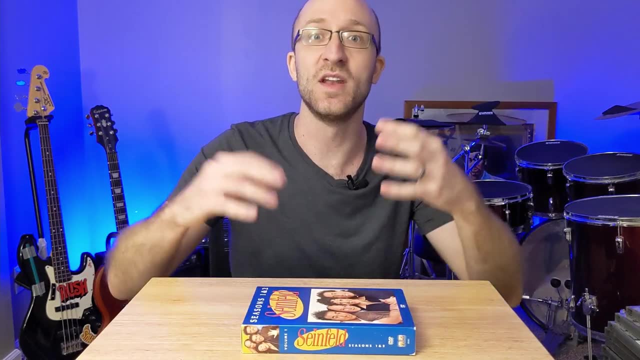 stack, then your program exits and finishes. But if Java is running your main method and it has that information for that method on the call stack, if inside that method it has to call another method, Java adds the information for that method onto the call stack too, And if that method calls another, 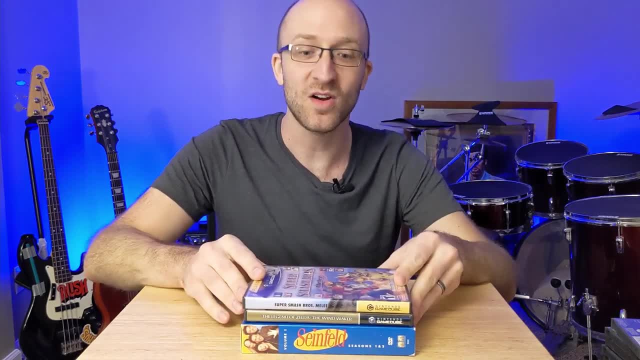 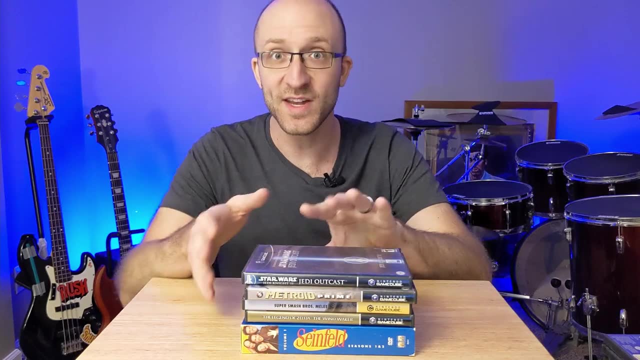 method inside of it. Java has to add that method that it calls onto the call stack too, And this keeps going and keeps happening, And that's why it's called the call stack. And that's why it's called the call stack The deeper that the method calls go. Now, when any of these inner methods 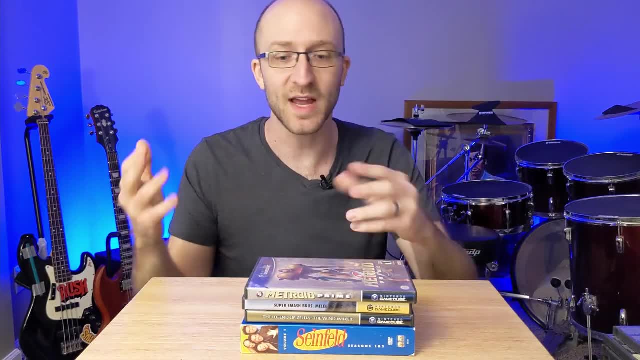 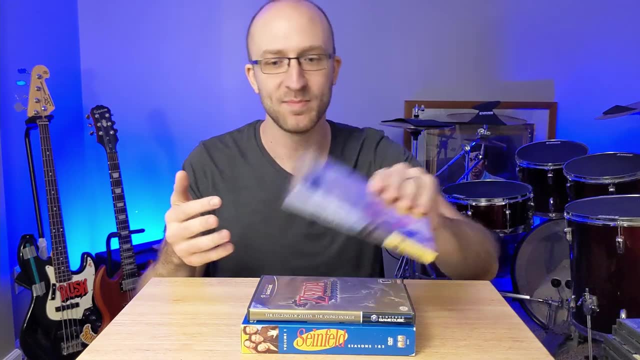 complete. Java takes the information for that method off the call stack because it's done with it. And while your program is running, Java keeps doing this, adding things and removing things from the call stack as methods get called from inside of other methods and as methods get. 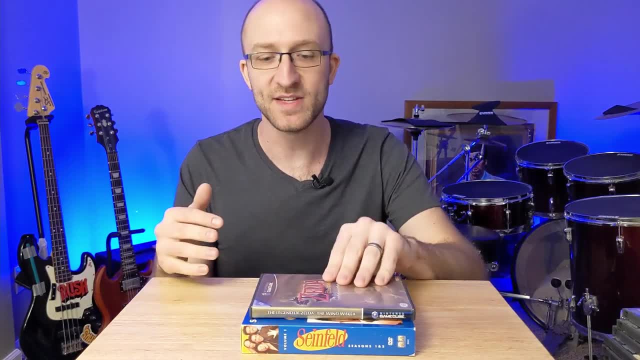 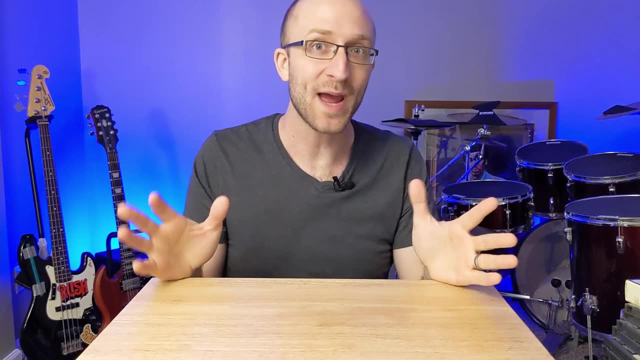 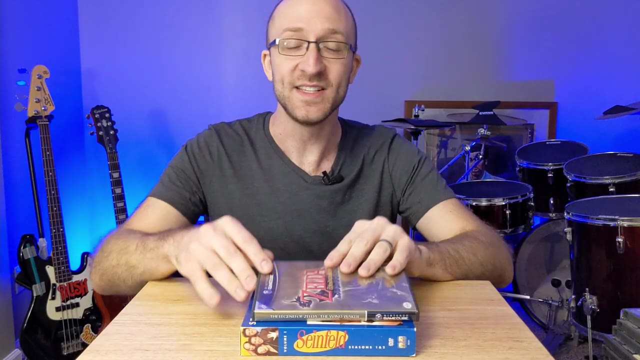 completed and things get removed from the call stack And it keeps doing that until it finally gets back to your main method and your main method eventually completes ending your program. But here's what happens with our recursion situation: First the main method is called and that info goes on the stack. Then the main method calls the. 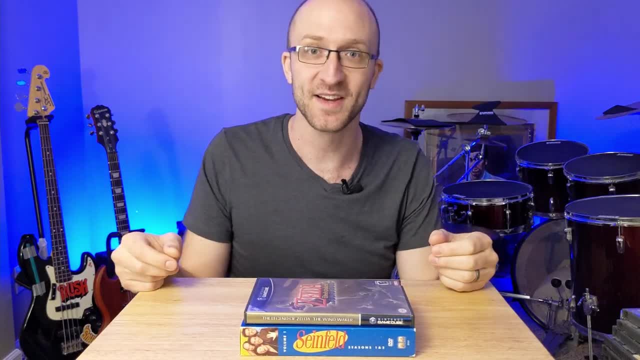 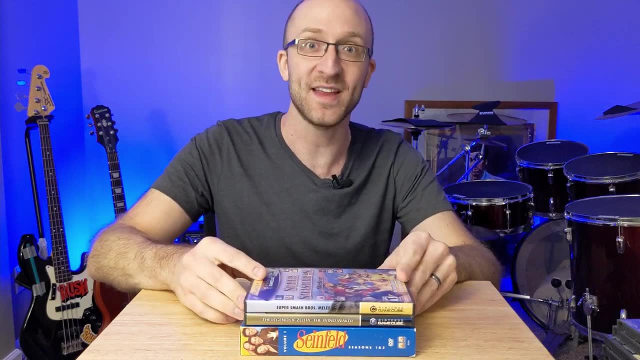 sayHi method and the information for that method call goes on the stack. But before this sayHi method finishes, it actually calls the sayHi method again from within it And the information for that call to sayHi gets added to the stack. You get the picture. The same method gets called. 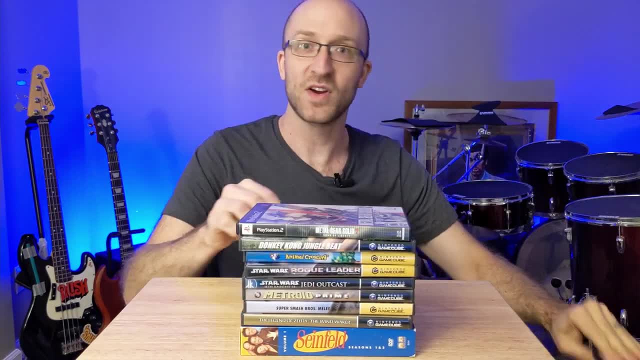 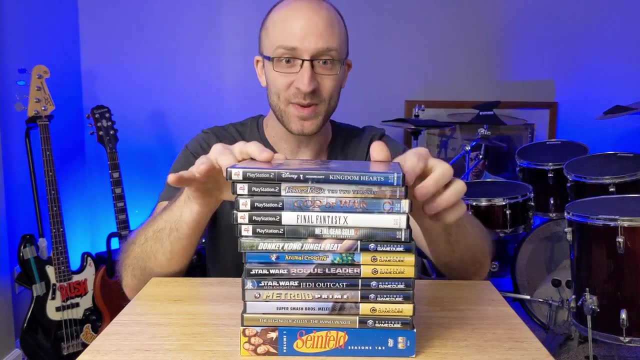 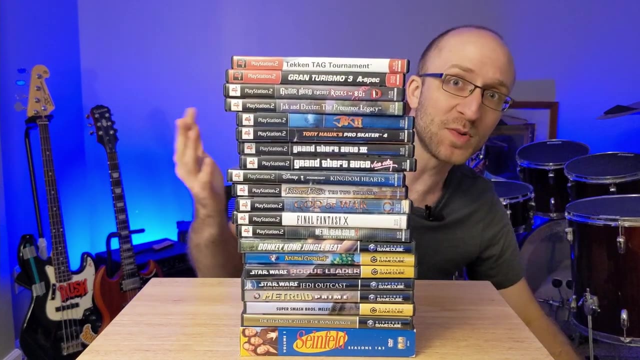 recursively, over and over and over again, and the call stack just keeps getting deeper and deeper and deeper. there's nothing in the program that will stop it from just continuing to grow. so it just keeps growing and growing. but the thing is, java only has so much memory allocated to this call stack. 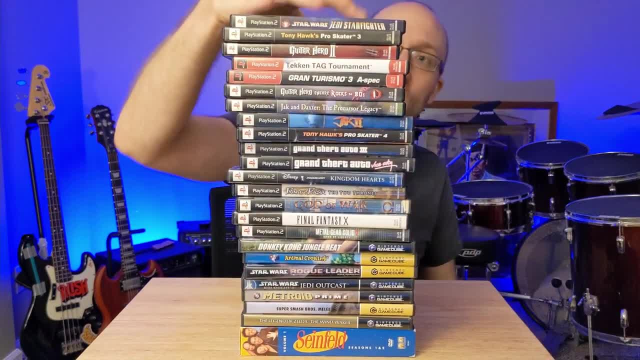 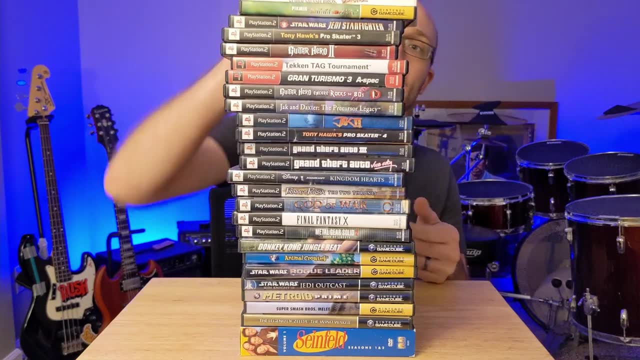 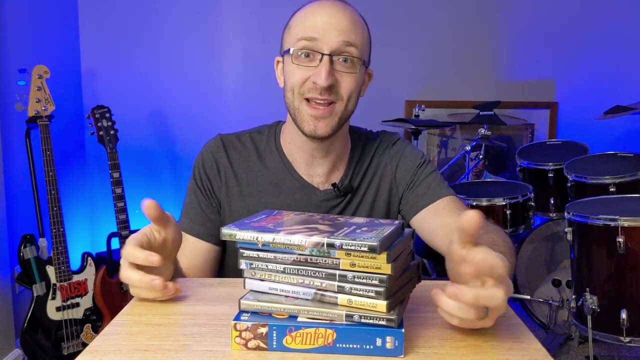 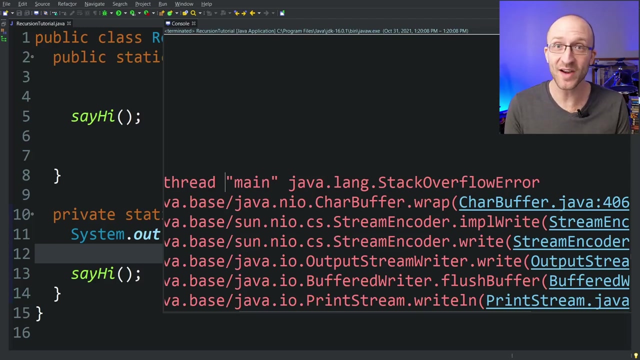 so if you just keep adding method call information over and over and over again to the call stack, eventually that stack just gets so huge that it overflows and you get a stack overflow error. makes sense. so does that just mean that recursion is terrible and every single time we try to use it our program is going to blow up with a stack overflow error? 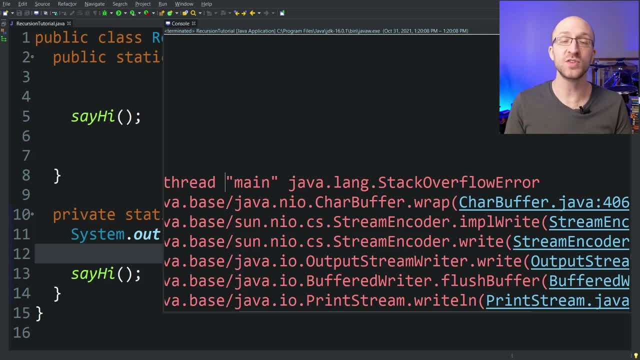 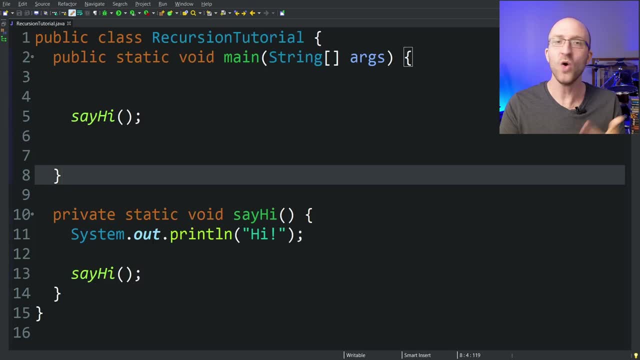 well, yes, unless you know how to code your recursive programs right so that that doesn't happen. the problem, of course, is that it just keeps calling this method over and over again recursively right and right now in the program. there's nothing that would ever stop it from making. 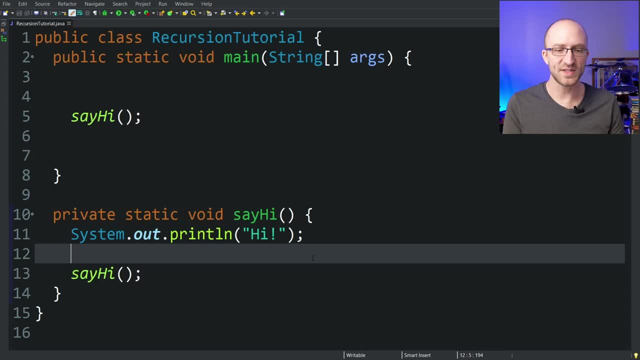 that recursive call over and over again. so what we need to do is have something so that this method stops calling itself recursively at some point. basically, you need an exit strategy. right, here's a simple way we can add something like that to our program. here let's add a parameter to our 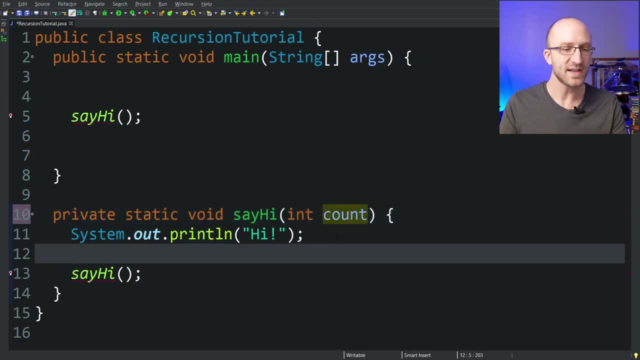 method, we'll make it an int and we'll just call it count. next, let's add a condition in our method after we've already printed high, so that if that count is less than or equal to one, we just return. so if the count is less than or equal to, 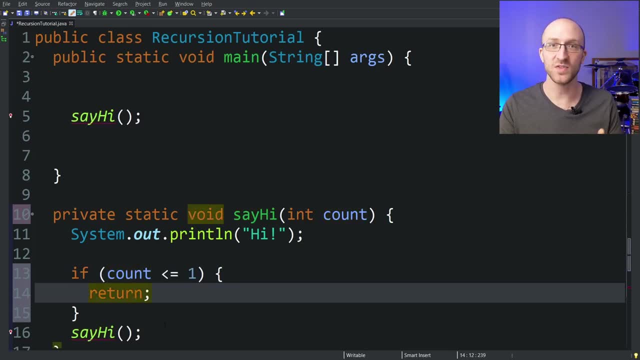 one, it will just return and exit the method and not recursively call say hi. but otherwise, if the count is greater than one, it will recursively call the say hi method. but when we call this method recursively, instead of just passing in the count that we received, let's pass in count minus. 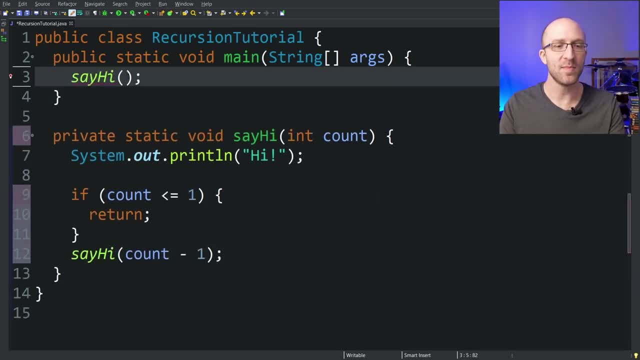 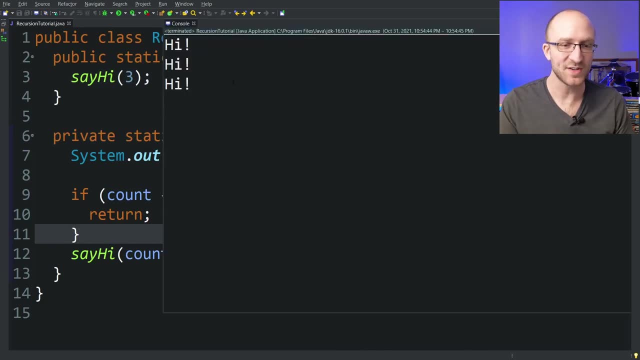 one and then up here where we're first calling the say hi method from our main method. let's just pass in three for the count. so now, if we run our program, we can see that it just prints out high three times and completes successfully. so let's walk through what happened there. so the first. 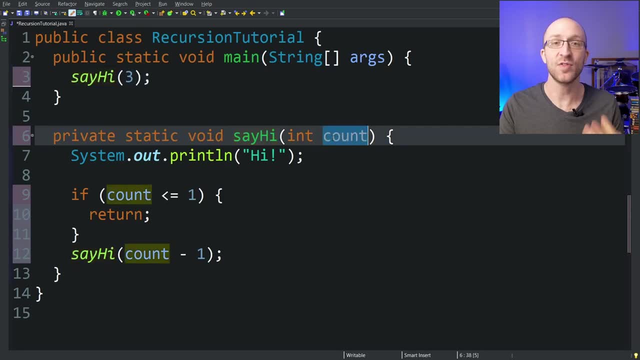 time that this say hi method is called it gets passed in a three for the count. it prints out high, the count is three, which is not less than or equal to one. so it skips this condition and calls the say hi method recursively, but it calls it with a count parameter of two that run of the method. 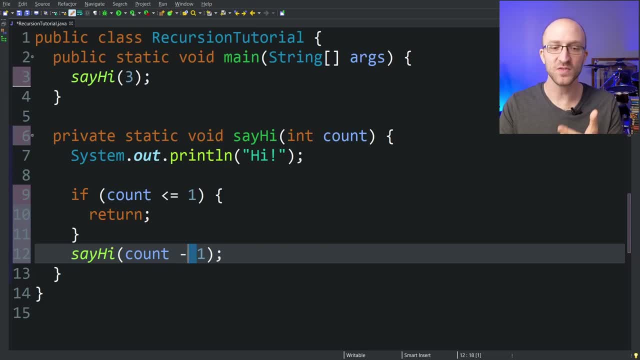 for the count. and three minus one is two, so this method is recursively called with a count of two. it prints out high again: two is still not less than or equal to one, so it skips this condition and recursively calls the say hi method again. but two minus one is one and it recursively calls the. 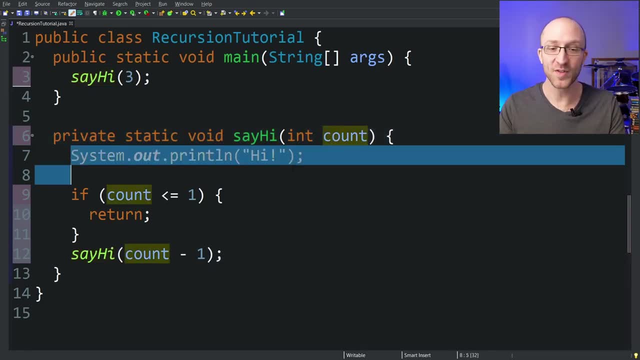 say hi method with a count of one, then that run of the method prints out high again, but this time the count that it received is one which is less than or equal to one, and so instead of calling the say hi method recursively, it just returns and exits that run of the method. so that run of the 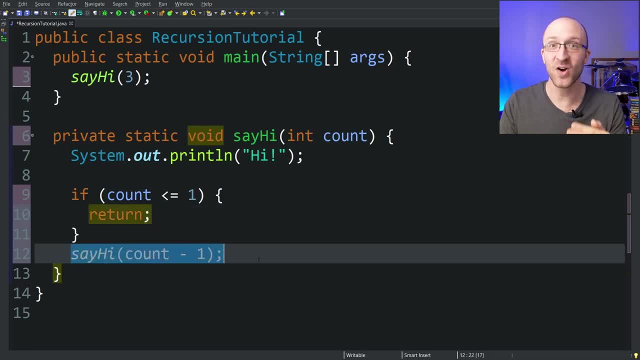 method returns back to the run of the method that called it recursively and since the recursive method call that that run made completed successfully, it will return as well up to the run of the say hi method that called it. and those method run completions keep bubbling all the way. 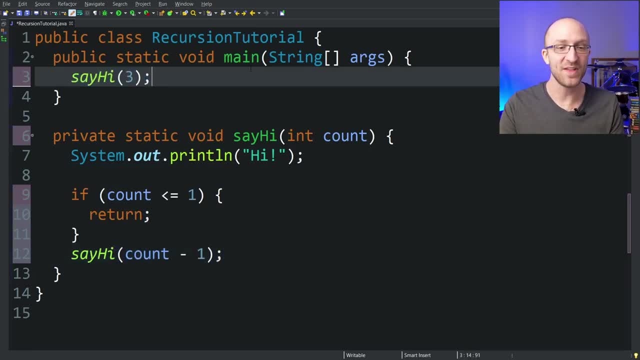 back up to the original call to the say hi method that was made from our main method and then, finally, this original method call is complete, which ends our main method and ends our program. so a recursive program doesn't have to die with a stack overflow error. if you have an exit strategy like this, there 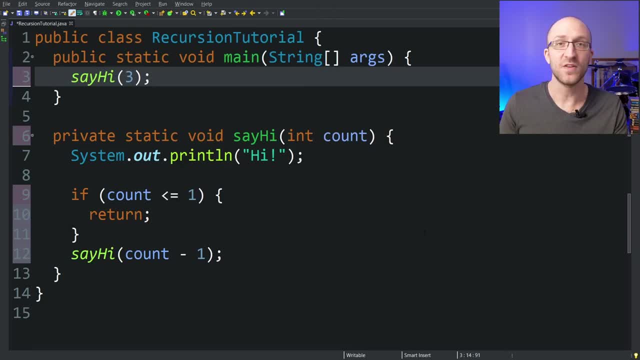 are a couple of parts of that exit strategy that we've implemented here. the first thing is called a base case. a base case is a condition inside your method where it can return without making another recursive call. that's the condition that your recursive calls eventually need to hit, so it 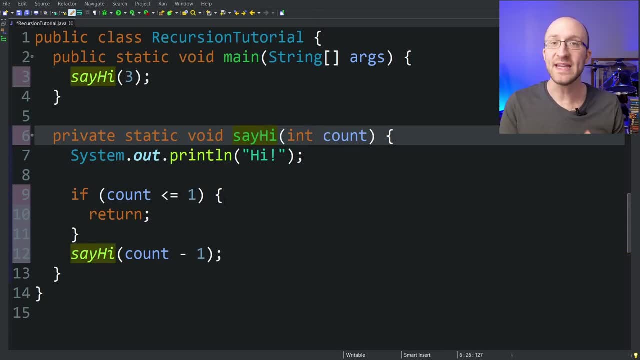 can return without controls in the run method and automatically that is returned to your original method. and this is the end of the reservation for the method. call language ret か, going deeper and deeper into recursion forever. You need a base case in your recursive method, otherwise you will always go into infinite recursion and your program will eventually. 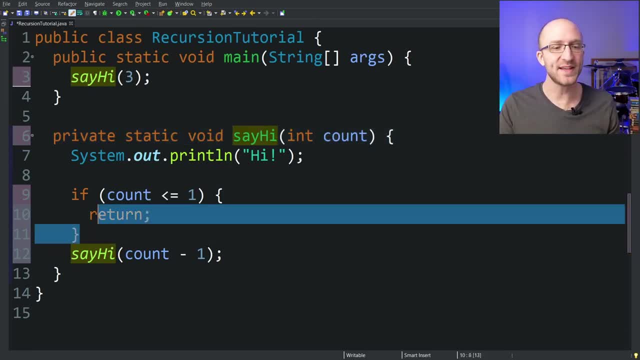 blow up with a stack overflow error In this program. our base case is here, where if the condition is reached where count is less than or equal to one, it just returns out of that method without making the recursive call to say hi. But the second thing you need is that in your method. 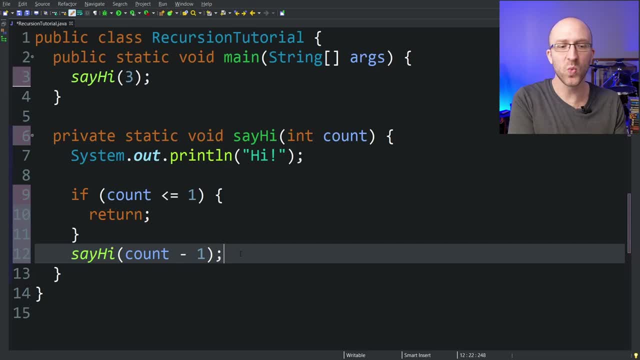 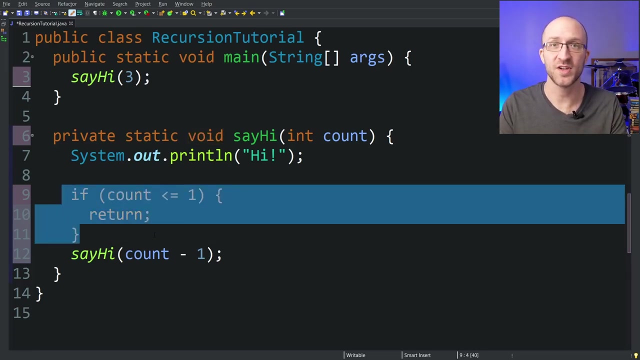 you need something that allows it to work toward that base case every time it recurses. So even if you have a base case like this, it doesn't matter if your program never actually runs into this base case. Your code needs to eventually get to this base case or you're going to get infinite recursion. 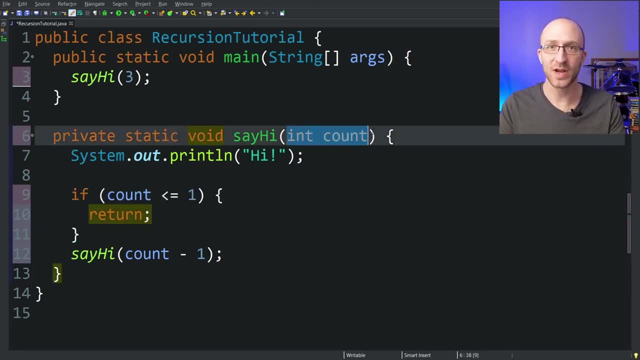 Now in our program that was done by adding this count parameter and by using count minus one as that parameter each time we call the say hi method recursively. So each time this method is called recursively it reduces this count by one. So no matter what number is passed into the initial say hi call. 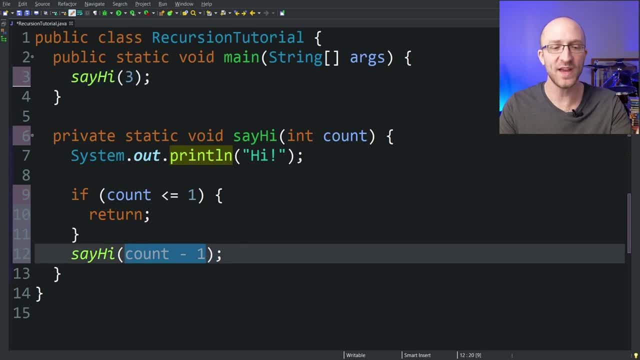 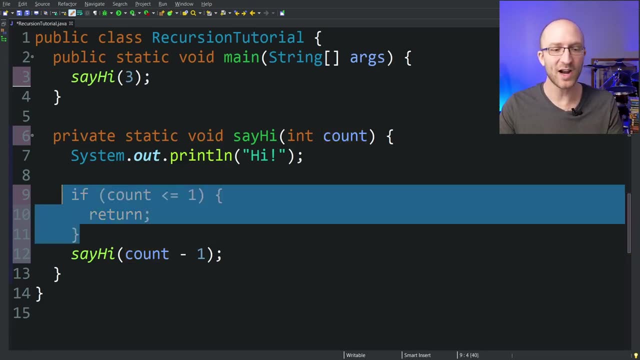 each time the recursive call is made, it gets reduced by one. So eventually it will reach the base case where the count is less than or equal to one. And when it finally does hit our base case, it returns without making the recursive call, which finally ends the cycle of recursion. So together, 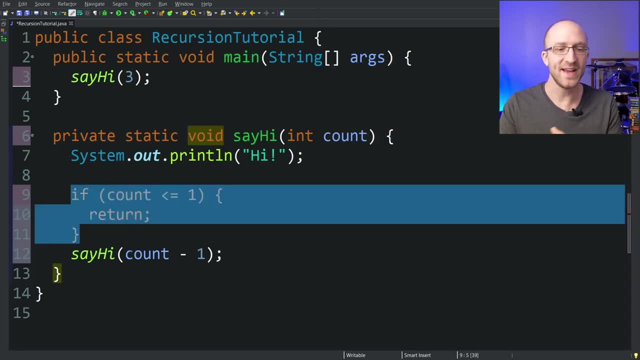 having a base case where we don't call the method recursively and having code that allows the program to work totally without the recursive call, Then we have to make it so that we actually have that building base case and we don't have to call the method recursively. So in order to get some rest and get the quality of the project, 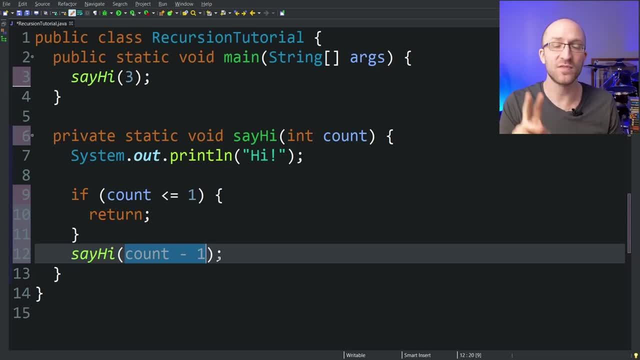 in the first place, we need to have a recursive algorithm where we canый make it so we don't get infinite recursion. So every recursive algorithm has to have those two elements in order to not get a stack overflow. However, I will note, even having those two elements doesn't absolutely. 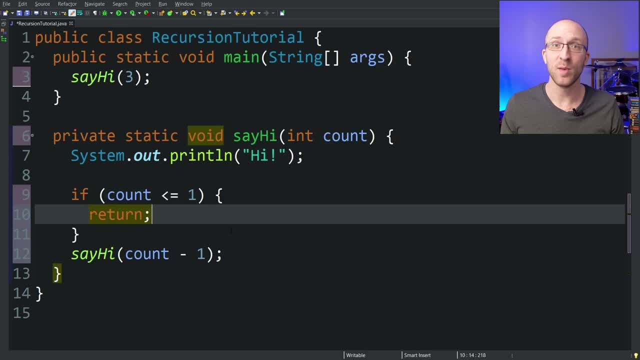 guarantee that your program will always finish before it gets a stack overflow. If it has to recursively call itself tons and tons and tons of times before it actually reaches that base case, you could still run into problems. For example, we could call our algorithm before the end of a star.